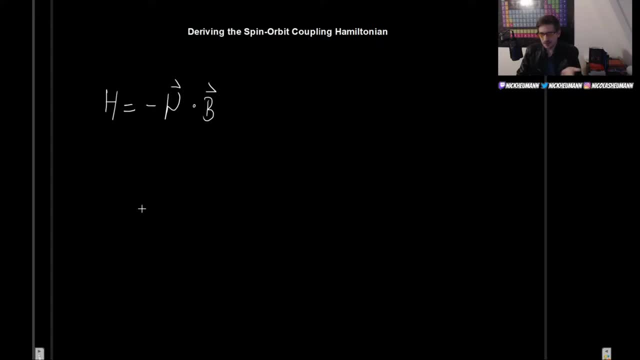 solve it by using the Biot-Savart law. Now, this is a quantum mechanics course, I'm not going to get into that. But the field that you get out of that is mu naught. i divided by two times r right, With r, the radius there. 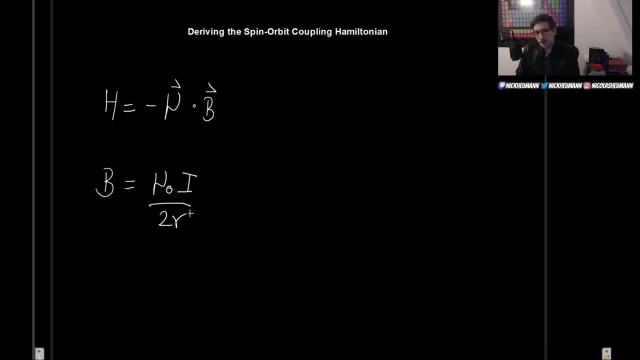 All right, so this is the magnetic field. okay, If you have any doubts, you know, just go back to electromagnetism, see how you find the magnetic field due to a ring of charge, and you have to use the Biot-Savart law and you will find this very formula. 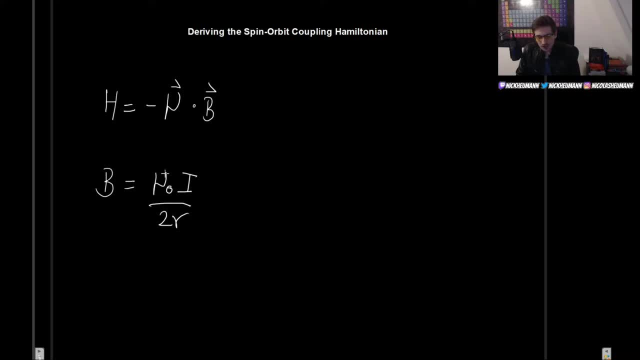 Okay, Okay, All right. so well, what do we have here? Mu zero, this is just a constant right, So no problem there. We don't really know the current, or do we So the current that flows through the ring? now let's. 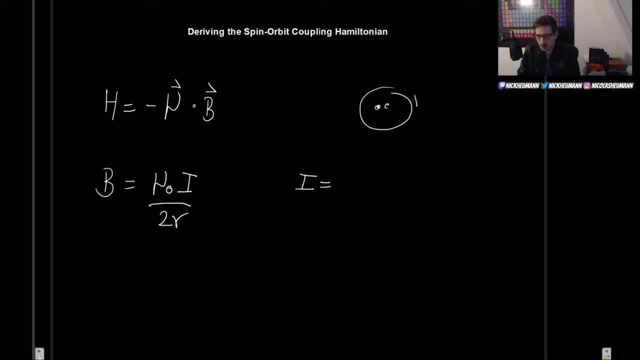 let's remember what is the ring. We have the electron orbited by a proton. So what we have here, basically, is going to be a charge q that moves around at some period. right, It will take it some time- that is the period of the rotation- to move around the electron, okay. 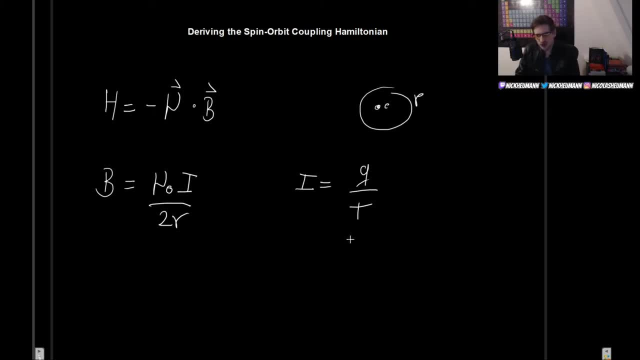 So we can actually use this. But the thing is that now we introduced a new quantity, which is the period, and we don't know what this is. So now we have to think of some other way to get rid of the period. Okay, I'm actually gonna maybe rewrite it. It kind of looks like a plus and I don't like it. Okay, so the way to? 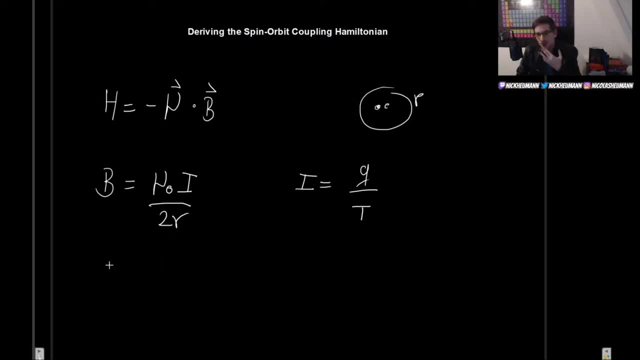 now get rid of. it is to think: well, we have circular motion and maybe, if we take a look at the angular momentum of the situation, right, classically speaking, this is all classically speaking- then, well, what is the angular momentum here? 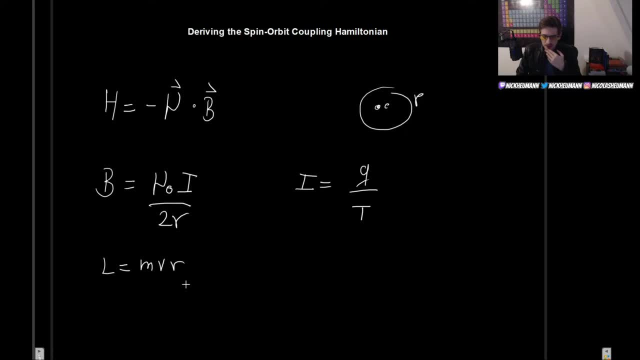 We are going to get MVR right. So what is the velocity in this case? Well, the velocity is simply going to be the distance that you travel divided by the time it takes you to travel That distance. So it's going to be- I'm going to move M and R here- 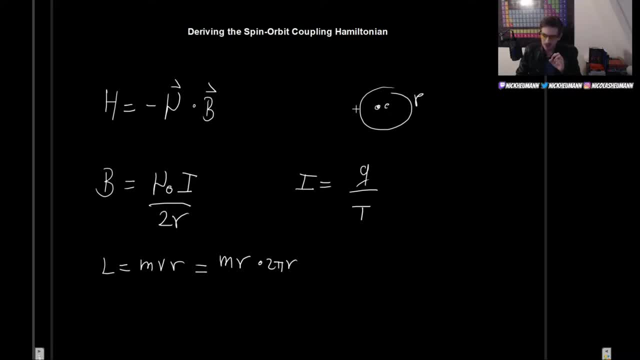 It's going to be 2 pi R right, the perimeter here of the movement divided by the period. So now we can find from this formula that the period is going to be 2 pi R squared times M and this is divided by L. 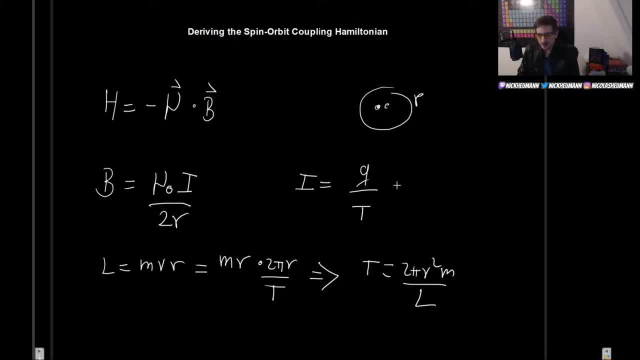 All right, cool. So we can actually now plug this into the formula for the current and we will have Q divided by, so let's maybe do it like this. So, since we are dividing by this, it's going to flip and we will have angular momentum divided by 2 pi. 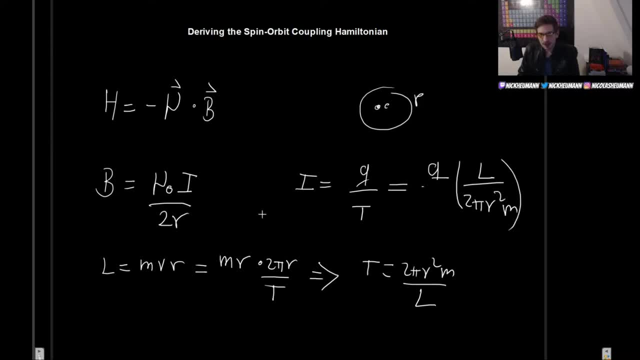 R squared M. And now we can plug this into our formula for the magnetic field. So the magnetic field is now going to be mu naught 2 R times this beast right there. So it's going to be Q divided by 2 pi R squared M. 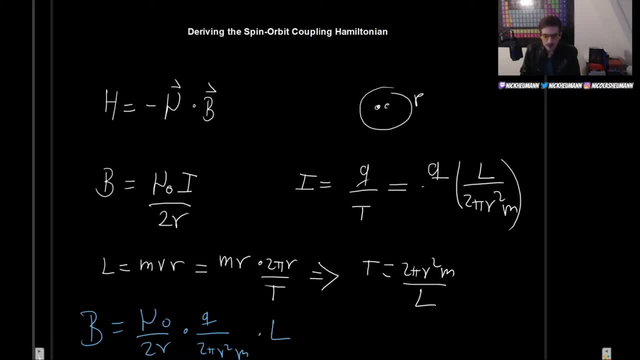 So the magnetic field is now going to be mu naught to R times this beast right there. So it's going to be Q divided by 2, pi R squared M times L. Now let me just move this to the new page, and we can now work on further simplifying this. 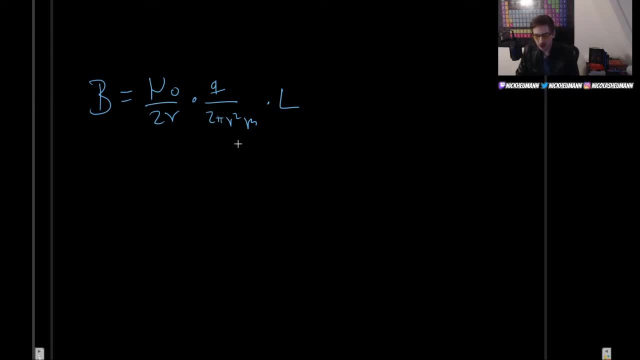 So there's a few things we can do. Of course, we can multiply everything through here, And there's also something very, very important, which is that we have this mu naught here, and it's not really imperative that we do it, but it's nice if we rewrite this not in terms of mu zero, but in terms of epsilon zero. 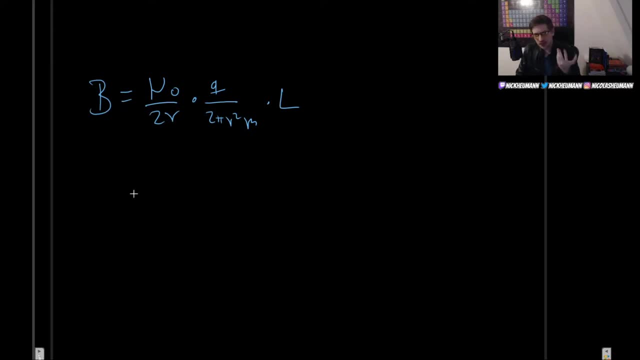 for example, and we know how mu zero is related to epsilon zero, because we know that the speed of light is going to be 1 over the square root of mu zero, epsilon zero. So from here we can find that. and if this confuses you, Well, I hope you saw this in the electromagnetic theory courses. If not, I guess you have to take the word for it for now. 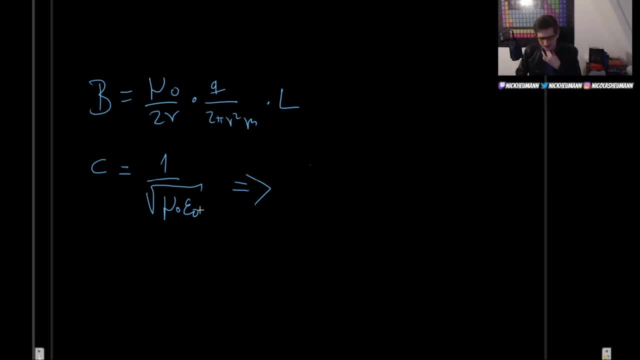 I'm sorry, I have a dry throat today, I don't know why. okay, so from here we can find that mu zero is going to be one over epsilon zero, c squared. so now let's just plug everything into the magnetic field formula, which is going to be- let's see one. 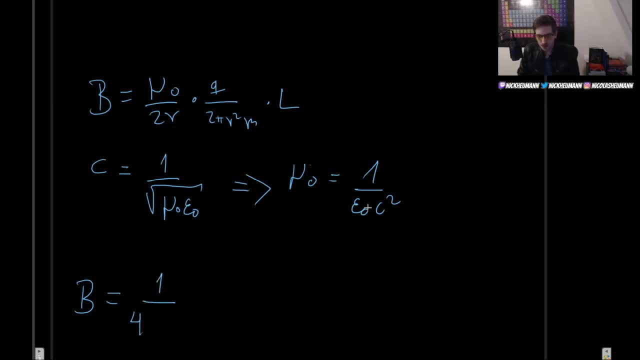 over. so here we have four, then we have this epsilon zero, and actually we have a pi, so let's write it as one over four: pi, epsilon zero, just to get the usual formula that we always see. and what do we have then? well, the charge is going to be e, so let's write it as e. 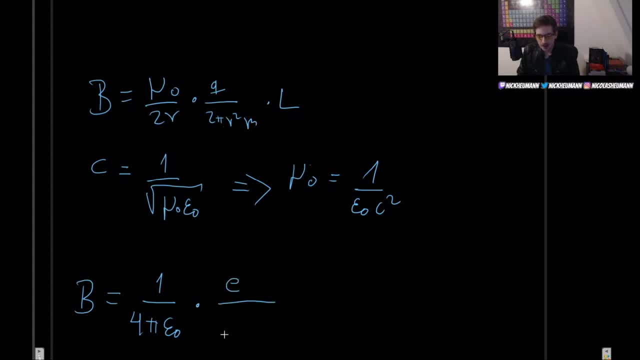 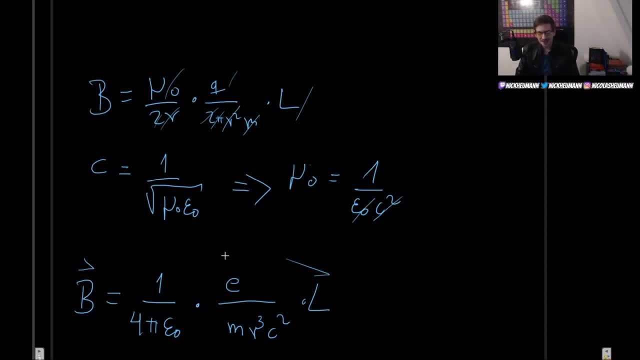 okay, we have solved the first part. next, let's now worry about the magnetic dipole moment. all right, so once again, we'll have to draw some of our knowledge from electromagnetic theory, and what i hope you saw in those courses is that the magnetic dipole moment of the of basically a ring, 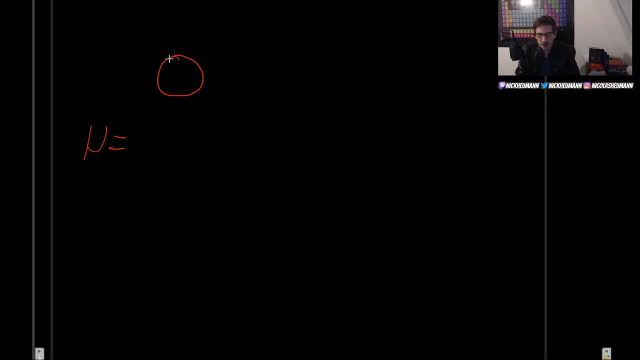 of charge, because we will have, now, looking at the electrons movement, it's basically going to be a ring of charge, right, and it's going to comprise a certain area and we'll have a certain current flowing through the area. so the way to find this amount, this dipole moment, is going to be the current times. 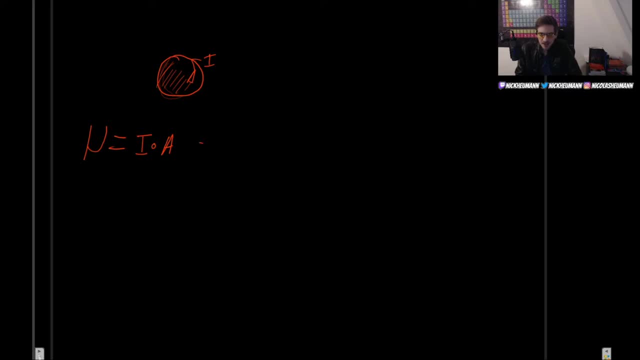 the area that it is moving around and, once again, we will these quantities we can easily find. so what is going to be the current? it's going to be the charge divided by the period, right the time it takes it to move around, and we'll have a certain current flowing through the area and we'll have a certain current. 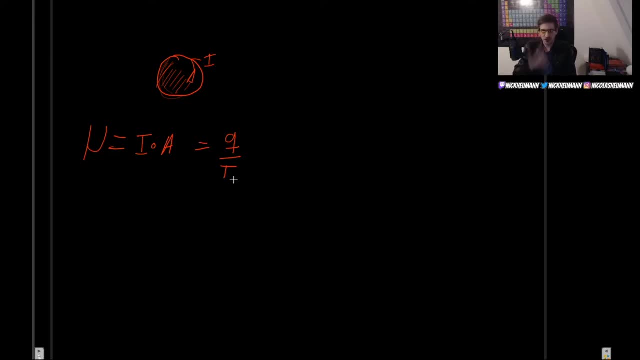 since the current is simply the charge that moves in a certain amount of time and the area is going to be pi r squared, all right. the thing is that now, once again, we are stuck with this annoying t, but we have a period here that we need to get rid of somehow, and once again since 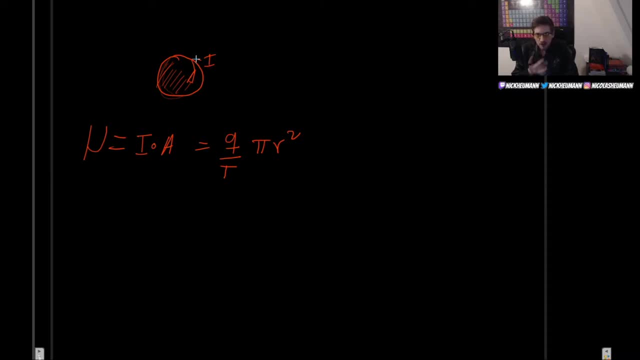 we're dealing with circular movement. let's now think of, well, angular momentum again, but this time we will deal with circular movement and we're going to talk about angular momentum again. now let's see if we can get into the Ward's line again and then we'll say that syncron tracked and he's currently going to be doing it. 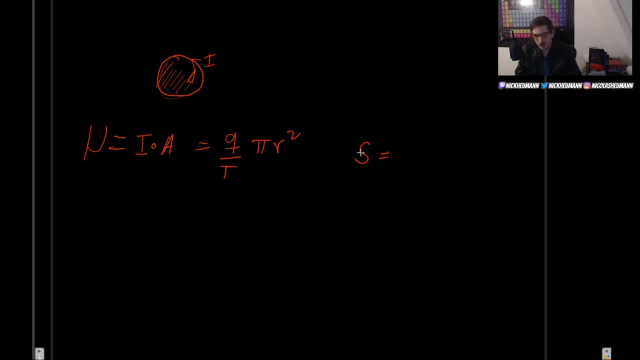 the other form of angular momentum. now, don't think of this as spin. i just don't want to repeat the letter l just yet, even though this will later be an analog to spin, of course. but for now we are only thinking of this, you know, in the classic sense. so classically we can think of this as: 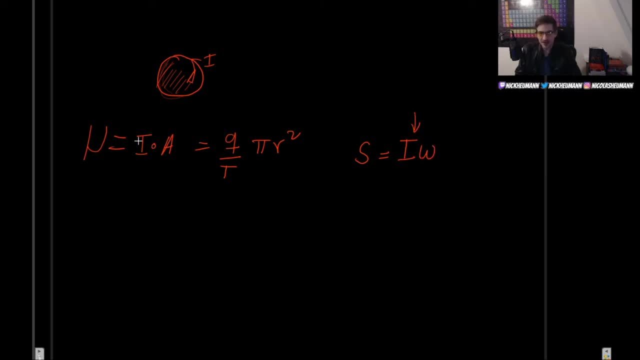 the inertia. now, let's not think of this as current, it's i2, which might be confusing, but it's going to be the inertia times the angular velocity. so what's this going to be? well, the inertia of just this, this ring, is going to be m? r squared, and the angular velocity, well, it's going to be two pi. 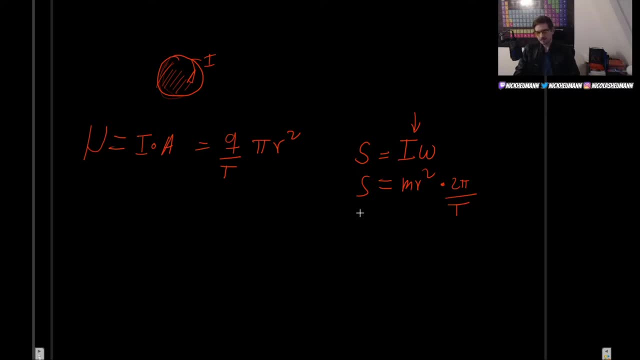 divided by the period, and this is why we did this right. so the period now shows up here, but we still need a way to relate mu and s, because if we just plug in the period, we can't plug in the period, then we're going to be left with S in of itself. 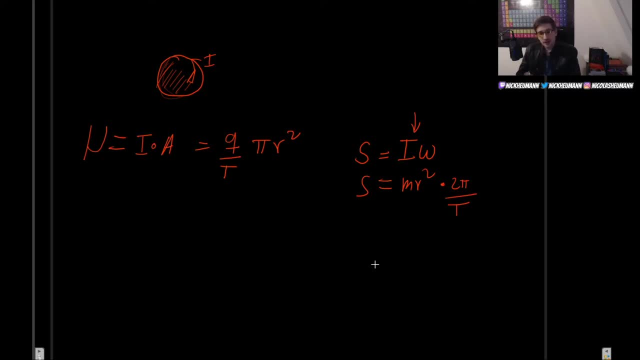 And well, there you could use, for example, the gyromagnetic ratio, which is simply the ratio of the magnetic double moment to the angular momentum. That's one way to go about it, And if you do that, let's see. 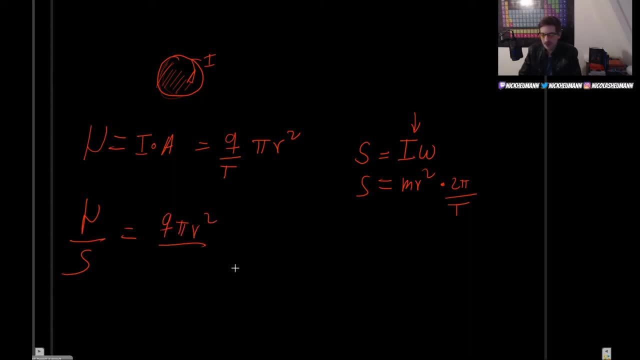 So it's going to be Q pi, R squared divided by M, R squared times 2 pi divided by T. Oh, and I missed this one. So the periods will cancel out and the R squareds cancel out. the pi cancel out. 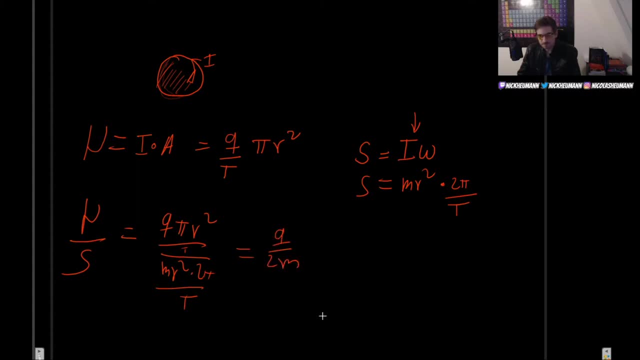 so we're left with Q over 2M. All right, And so we know that now mu over S is this amount. Thus, simply, mu will be Q over 2M times S. Okay, great. The thing is that we did this classically. 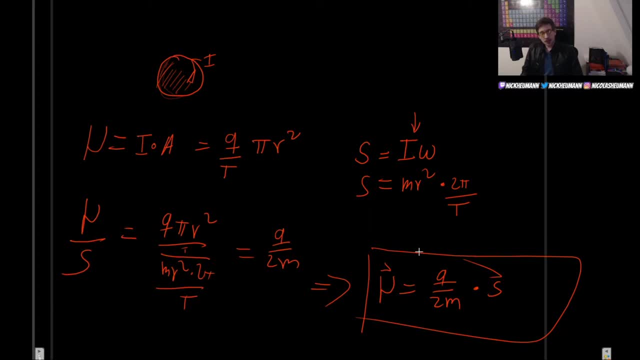 Why didn't we use a quantum mechanical approach? Because unfortunately, we do not have the tools yet to deal with this. If you're dealing in relativistic quantum mechanics, which is an entirely different formulation, you can actually do this calculation and we will find that the real magnetic dipole moment here is not what we just found. 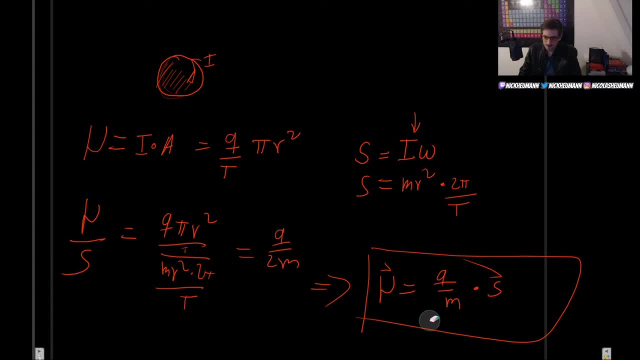 but it's actually twice this amount. So mu is going to be this. So this is what we will now plug into the formula for the Hamiltonian. So the Hamiltonian H is going to be minus mu times B. And well, let's now summarize our results. 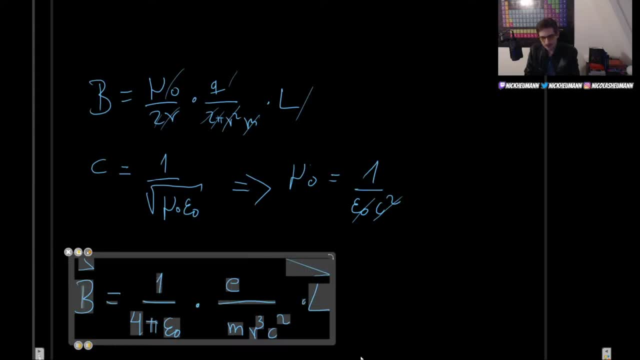 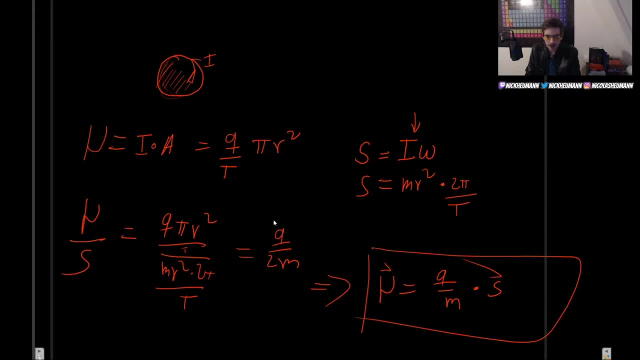 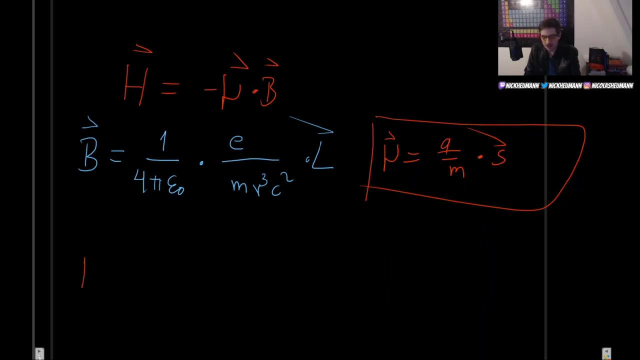 So B- was this right here, Maybe just put it there. And B And mu was this. So now let's just put everything into the Hamiltonian. So the Hamiltonian is going to be minus. So now comes Q and M, But Q is simply going to be minus E. 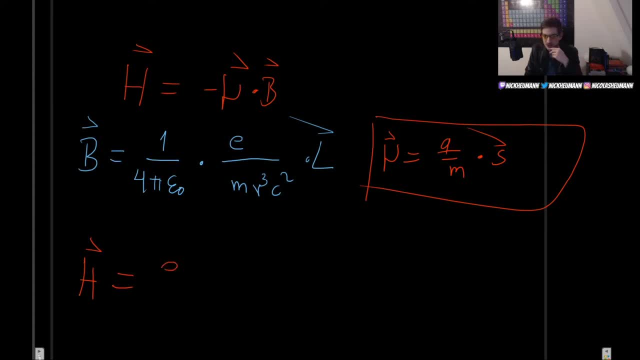 So it's actually going to be minus, minus, So it's going to be a plus sign. So we get E which, considering this, will now be E squared divided by 4 pi, epsilon zero, And then we have well, one over. 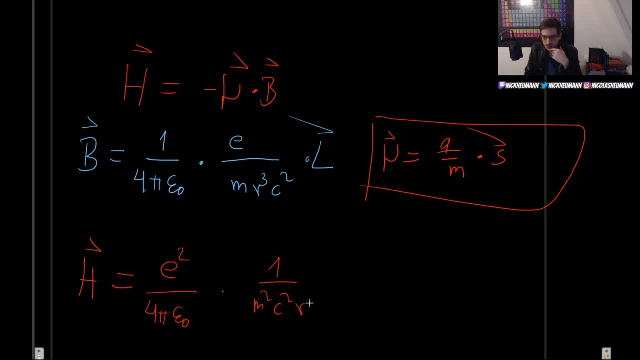 Now M squared, C squared, R, cubed, And then we get times, S dot, L. All right, So this would be the Hamiltonian. But there is one more issue that we have to introduce because of the fact that we did a classical approach. 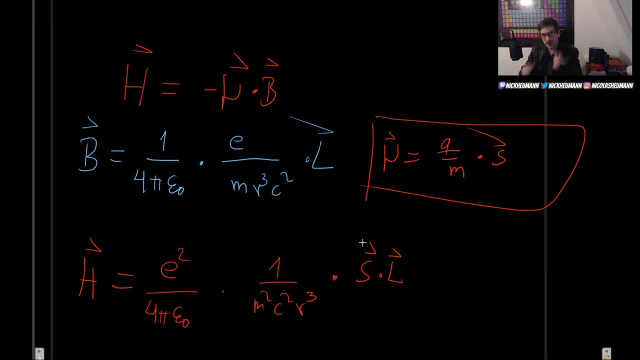 because we did not have the tools to solve this in a more sophisticated way, And that is that we consider this to be an inertial system, When it Actually wasn't. So that means that there is a factor that we need to introduce to correct our result. 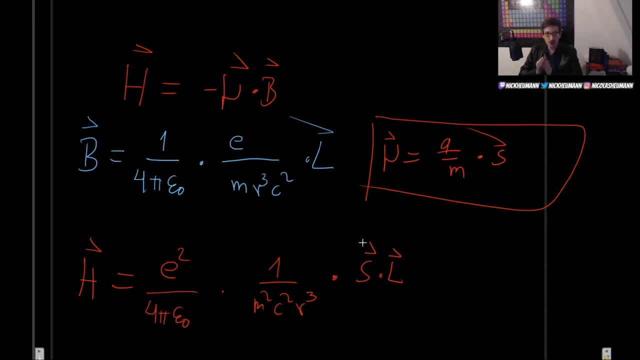 And that is a factor of one half, And that is due to a phenomenon called the Thomas precession, which is very interesting. We might maybe make a video about it if you are interested later, But for now it isn't really pertaining to the topic. 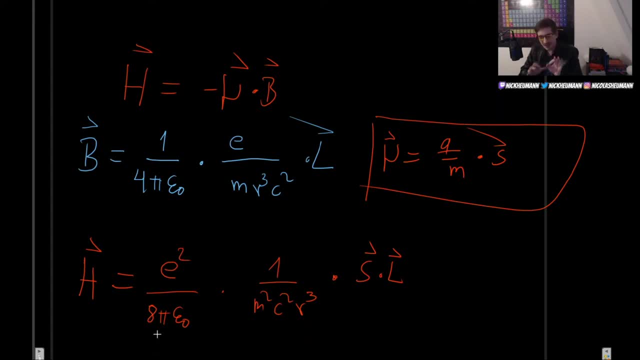 So we can leave it at this. So this is actually the Hamiltonian. This is what we can now use to find the fine structure of hydrogen, At least another part, the part that we call the spin-orbit coupling. There is something else that we could do, though, to maybe go a bit further. 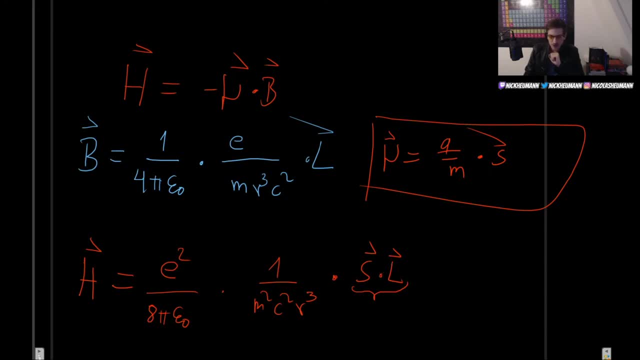 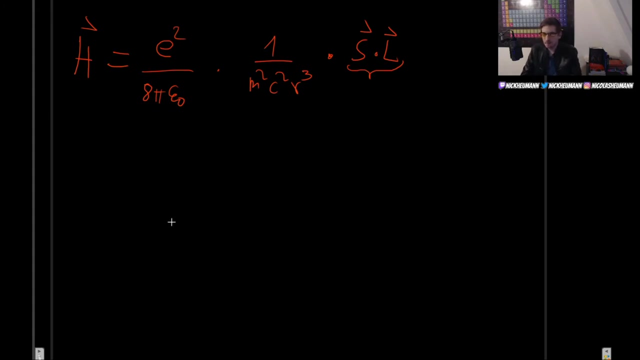 And it is that we have S dot L. So let's think of the situations that we will encounter. I'm going to get rid of this And just move it around. So the thing is, when we are dealing with some problem, we are going to be in the situation that we are dealing with. 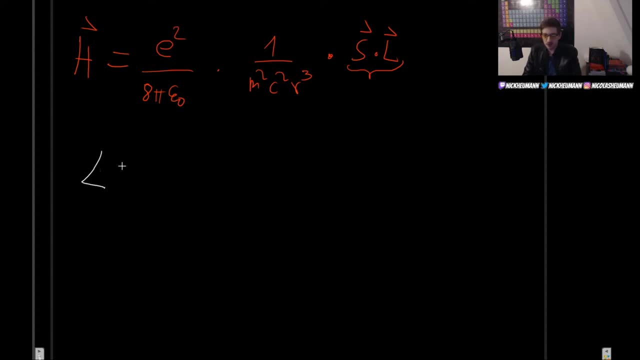 We are going to be in the situation that we are dealing with. We are going to be in the situation that we want to find some expectation value, So we are going to have some wave function sandwiching our Hamiltonian right, The way we always are. 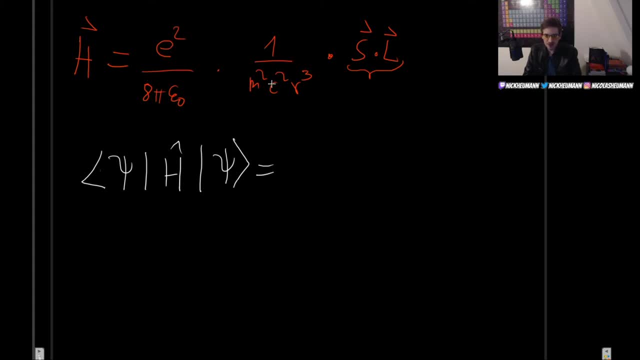 And just for simplicity, let's call all of these constants in front alpha or whatever you want, right? So we're going to have some alpha which can come out of the expectation value. Then we have psi, And then we have S, dot, L over R, cubed. 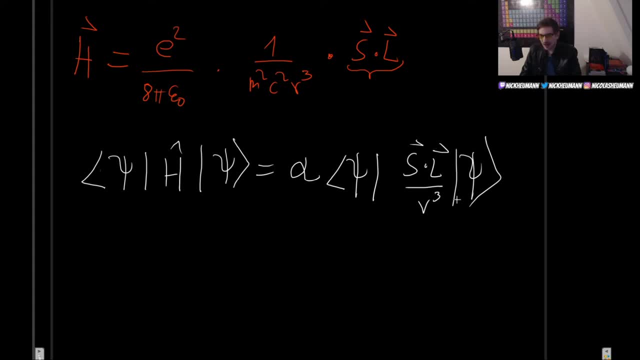 All right. So what is S dot L acting on psi? Well, what is S dot L Now, since we are dealing with quantum mechanics, once again, we're going to have to make the distinction between S which, if we go back, we were actually mimicking or kind of interpreting spin in a classical way. 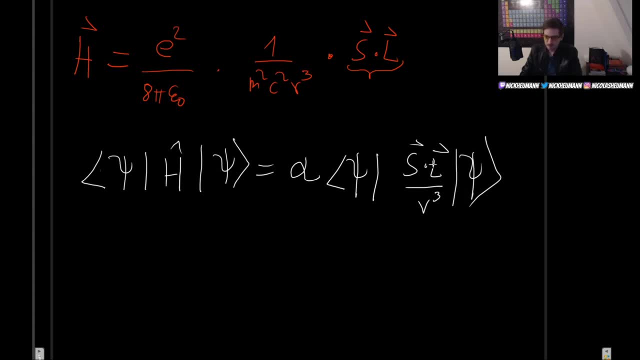 And L is just the angular momentum that we're used to. So we can remember that we had another amount, which was this total Angular momentum that we saw at the end of the first course of quantum mechanics, which was the sum of the spin angular momentum, or actually the normal angular momentum and spin angular momentum. 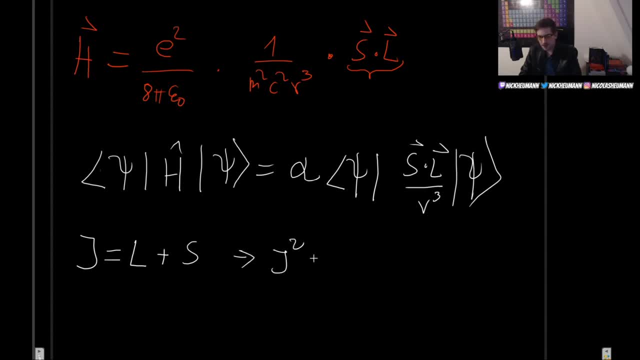 So if we were to consider, for example, the square of this amount, we would get L squared plus two L times S or S times L. they commute, so it's fine plus S squared, And from here we can solve for this quantity. 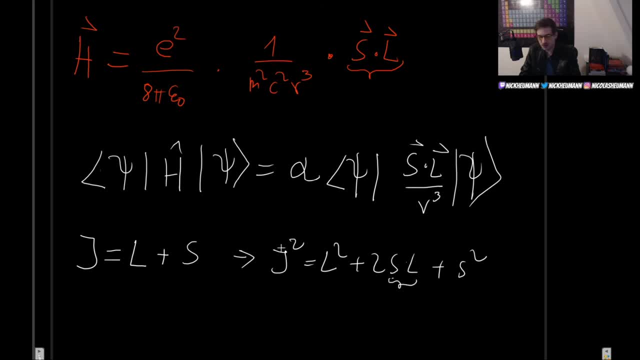 And in fact just S times L. we don't need the two, So S dot L. I kind of dropped all of the hats here because I'm lazy, All right. So S dot L is going to be one half of J squared minus L squared minus S squared. 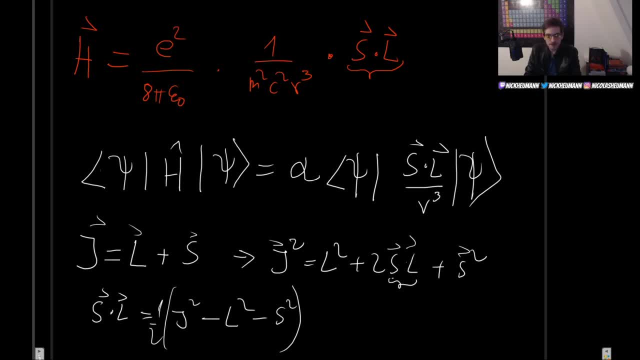 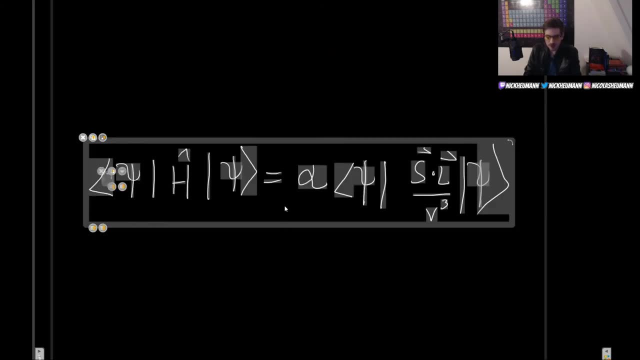 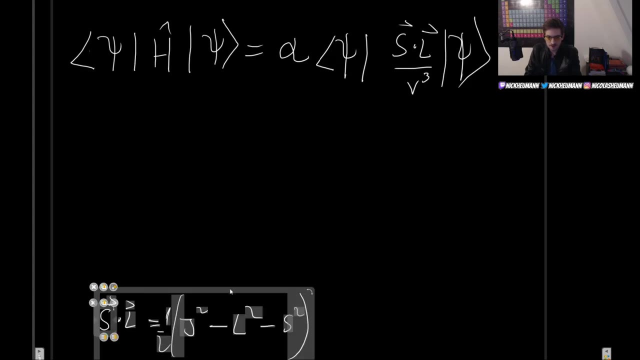 And we can now plug this in here. Um, maybe, let's how am I going to do this? Maybe, just like this, I'm going to copy this Onto the next page and then go back for our result. All right, 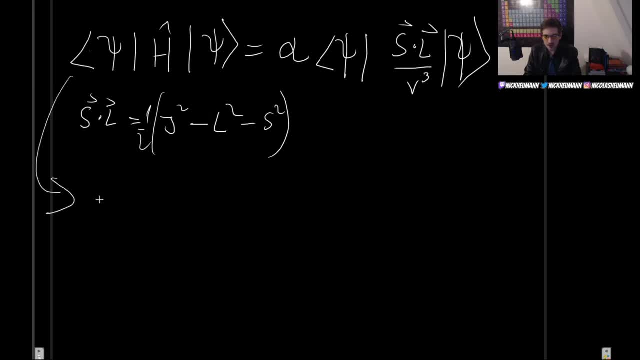 So now let's plug this in, So we get that this thing right here is going to be all of our constants, which I named alpha- once again because I'm lazy- times one half which we actually can pull out: J squared minus L squared minus S squared R, cubed. 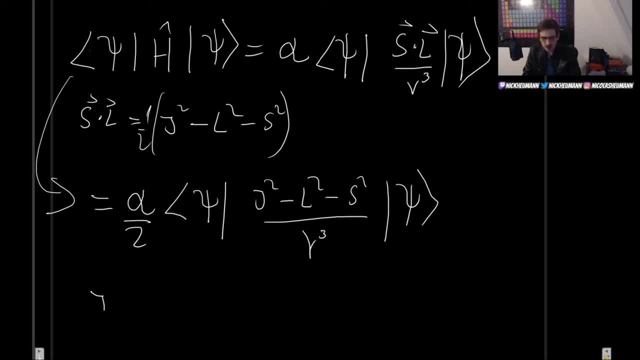 And all of this And all of this is acting on Psi. but what was J squared acting on Psi, for example? now, this was simply J J plus one right, And L squared acting on Psi was L L plus one. If this confuses you, I suggest you go back to the end of the lectures on angular momentum in the first course of quantum mechanics, because this is going to be very important in the next sections. 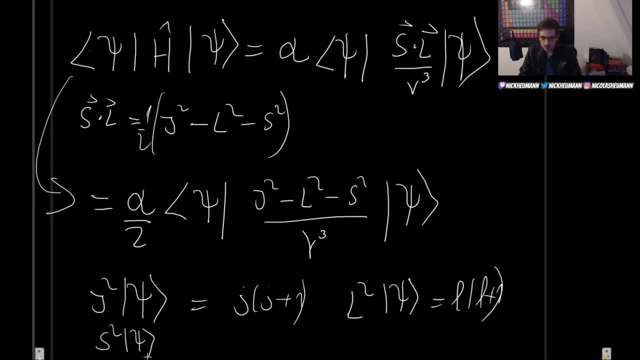 And similarly for spin S squared. We had this: acting on Psi was S S plus one. So using this, we can now rewrite what we just found. So this expectation value is going to be alpha over two Psi And then we get J. actually, I don't think I needed that parentheses, but I guess it doesn't matter. 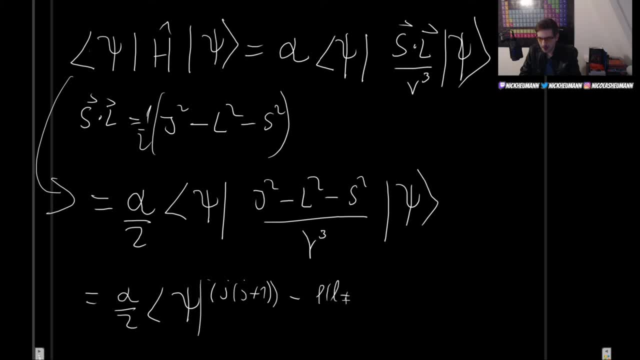 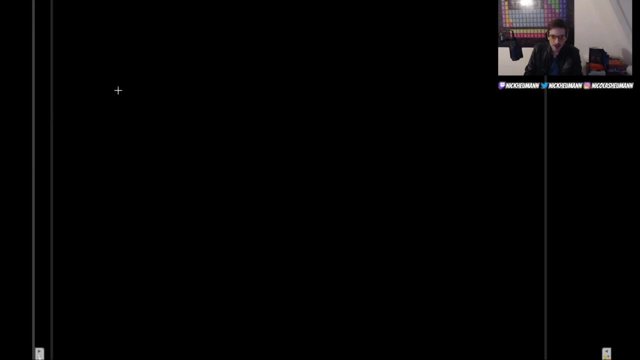 J plus one minus L, L plus one, Okay, One minus S, S plus one divided by R cubed, And we actually, um, didn't really this, we can now just pull out. So we would get that, this expectation value of the Hamiltonian, which we can call spin orbit. 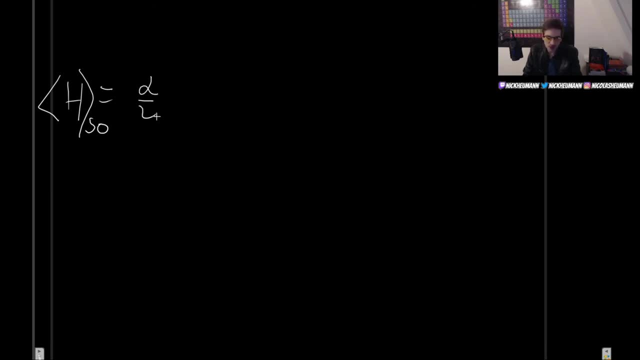 This is going to be now, well, alpha over two, all of our constants, which I guess I can once again write, which I forgot of course. um, it's E squared eight, pi, epsilon zero. I need to continually check because I have a bad memory: one over M squared, C squared. 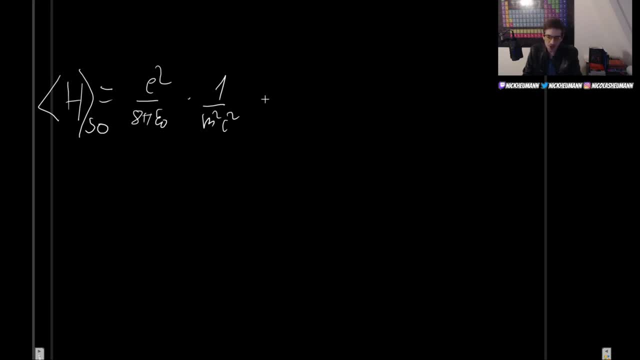 Okay, Times, I will. And now we add, of course, what we just found. So times: it was a J squared and J, J plus one, sorry, minus L, L plus one minus S, S plus one times the expectation value. So this is the equation of one over our um. okay, um here. one over R cubed.